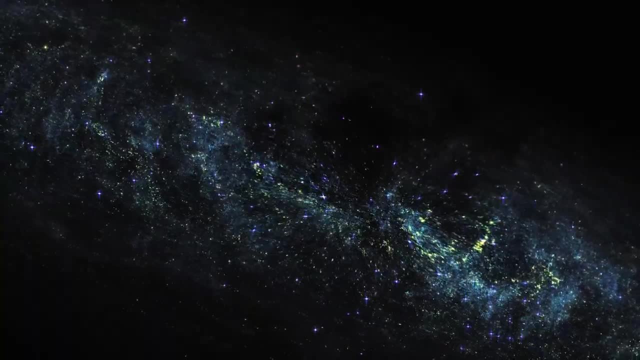 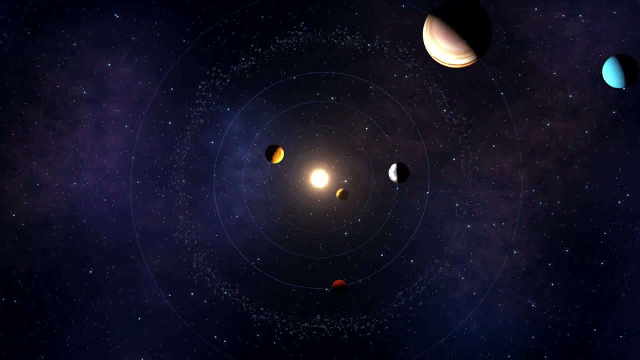 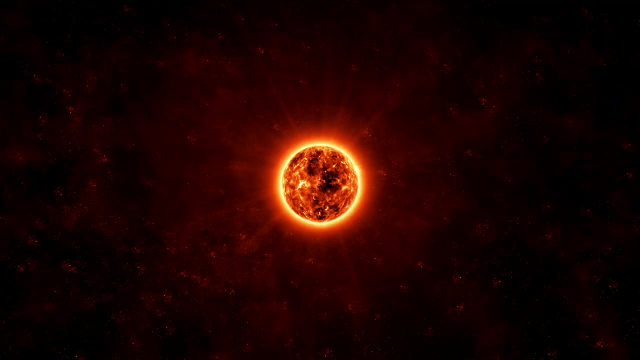 existence. Panspermia raises exciting possibilities for the spread of life throughout the universe. It suggests that the building blocks of life may exist in many planetary systems, increasing the chances of habitable environments. By studying the characteristics of extremophiles on Earth, organisms that thrive in extreme conditions, we gain insights into the potential. 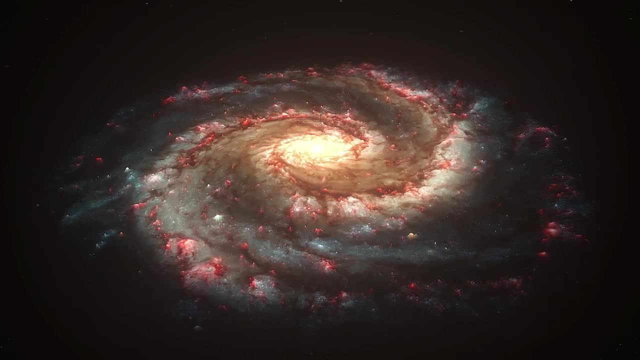 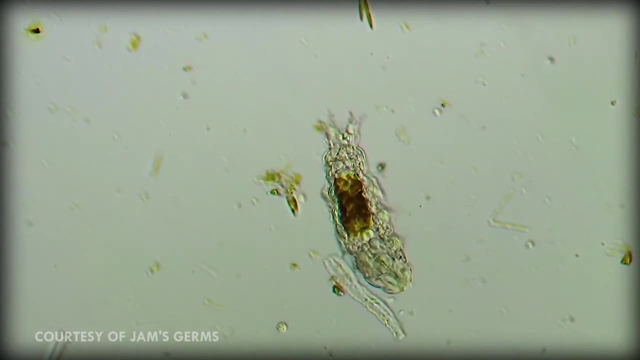 survival mechanisms of life in space and its ability to withstand cosmic journeys. These resilient microorganisms, known as extremophiles, are the most resilient microorganisms in the world. They are capable of surviving in extreme conditions such as high temperatures, radiation or the 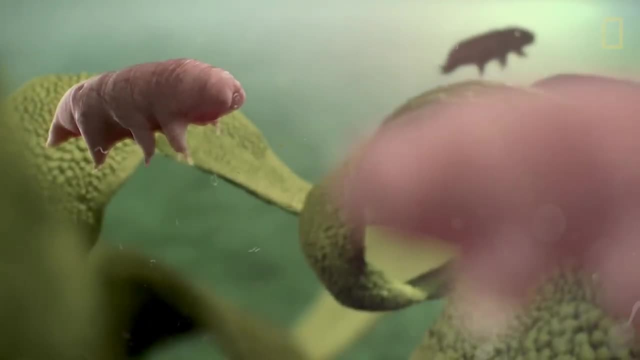 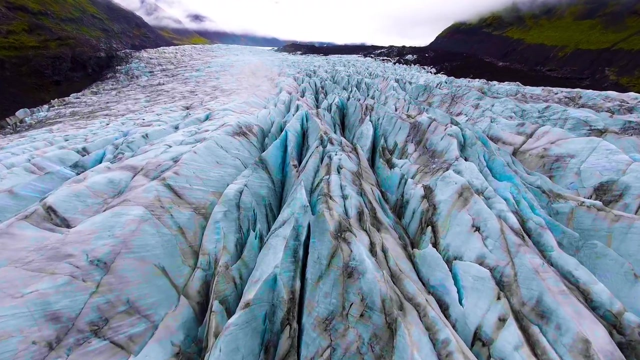 vacuum of space. Extremophiles have been found thriving in the harshest environments on Earth, including deep-sea hydrothermal vents, acidic lakes and even Antarctica's dry valleys. Their existence raises intriguing questions about the limits of life's adaptability. 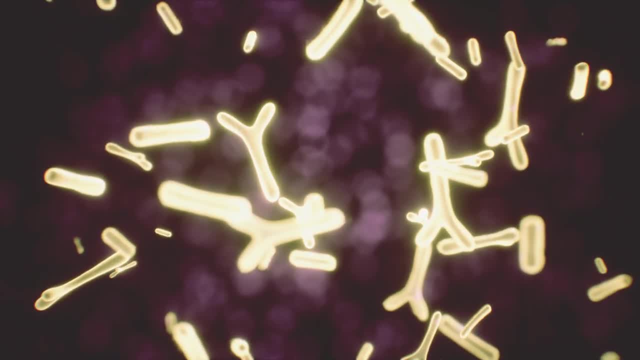 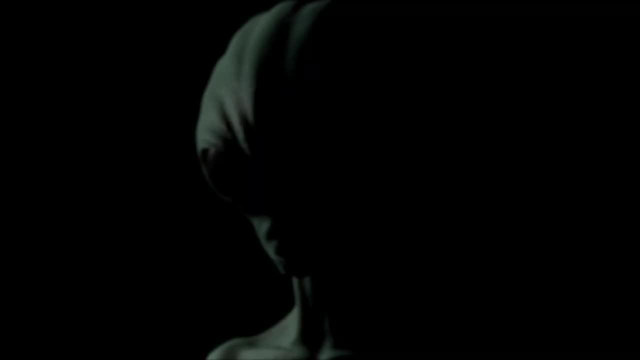 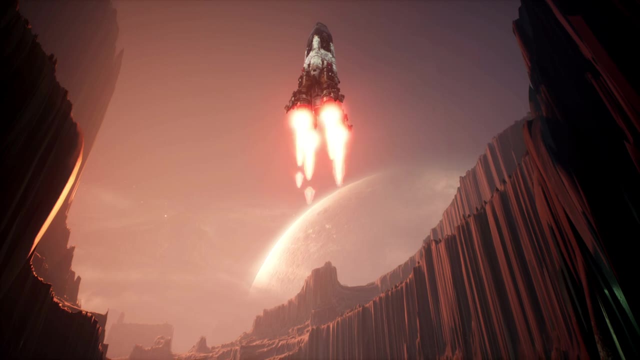 Panspermia suggests that if extremophiles can survive in extreme environments on Earth, it is plausible that similar microorganisms would survive in the harsh environments of similar organisms, could withstand the challenges of space travel and potentially seed life on other celestial bodies. panspermia expands our perspective, not only considering the origin of 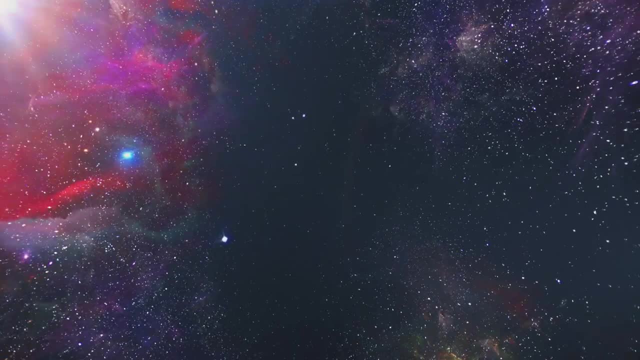 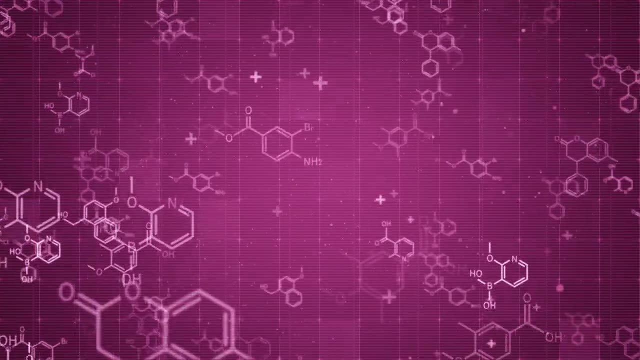 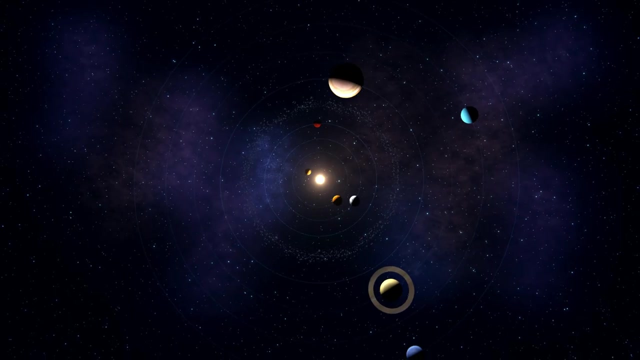 life on earth, but also contemplating the possibility of life spread throughout the cosmos. the discovery of organic molecules and building blocks of life on comets, asteroids and even moons such as enceladus and europa fuels the idea that the ingredients for life are present in various 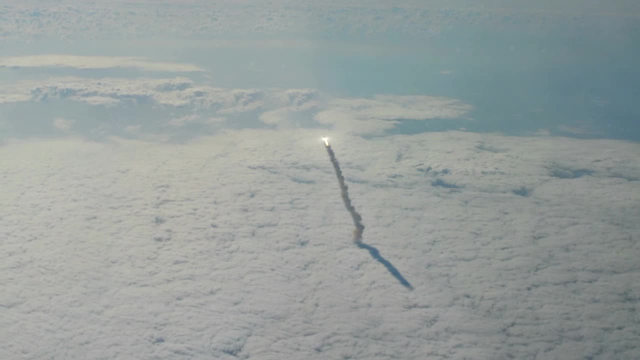 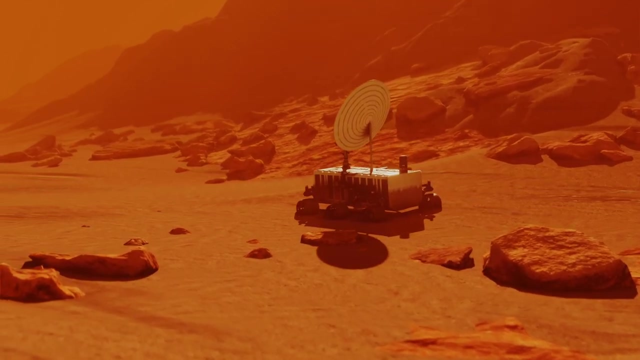 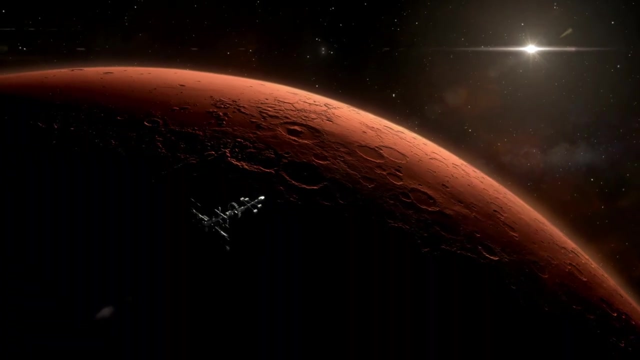 corners of our solar system. space missions like the rosetta mission and upcoming missions to europa and mars aim to investigate these extraterrestrial environments and search for potential signs of past or present life. the detection of glycine in the coma of comet 67p. 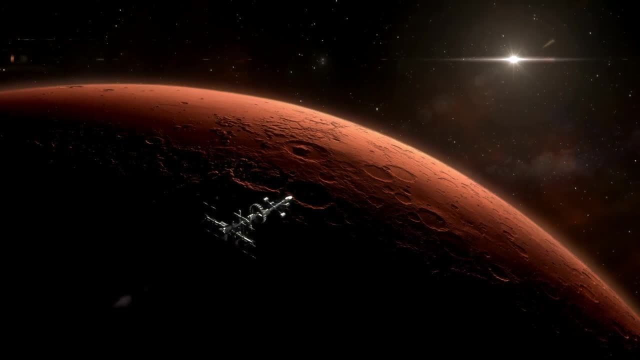 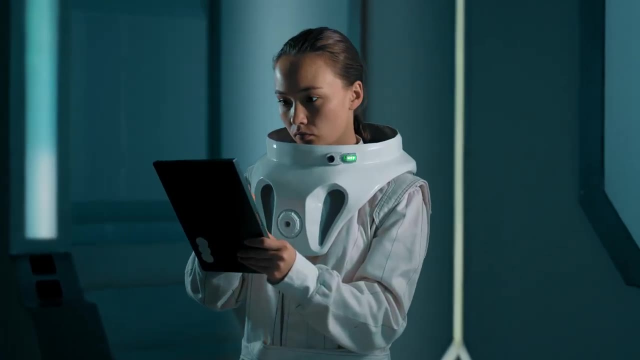 slash churyumov gerasimenko during the rosetta mission was a groundbreaking discovery that strengthened the case for panspermia. glycine is an amino acid, a fundamental building block of protein and amino acid that is responsible for the production of amino acids and amino acids. 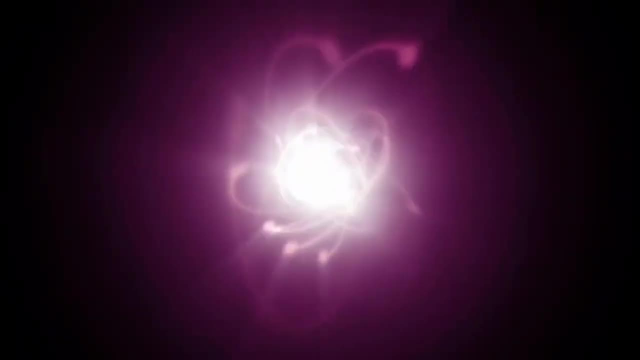 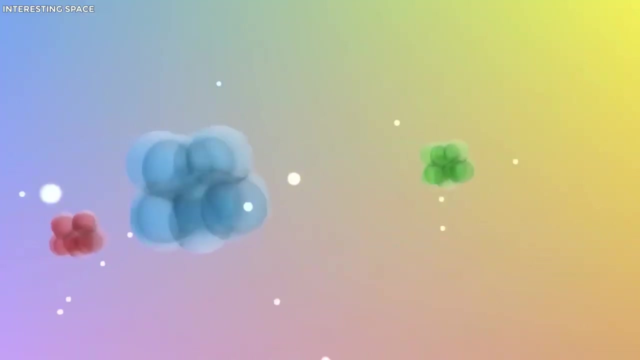 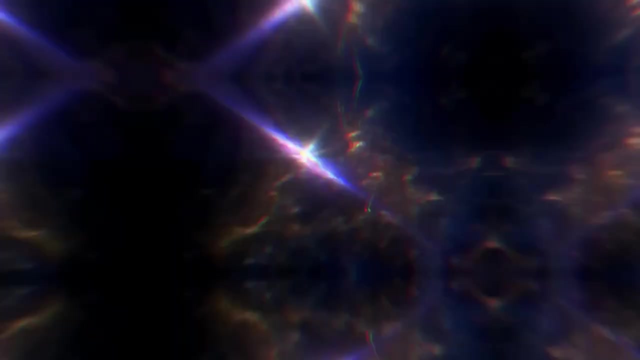 and a key component of life as we know it. its presence on a comet provided concrete evidence that organic molecules necessary for life can exist in the depths of space. this finding opened up a multitude of intriguing possibilities. if comets, which are thought to have formed billions of years ago in the early solar system, carry organic molecules like glycine, it suggests that 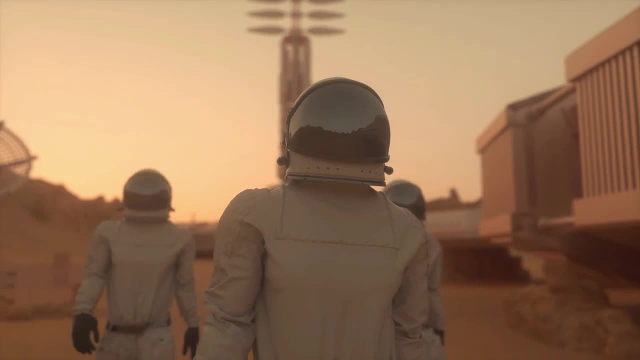 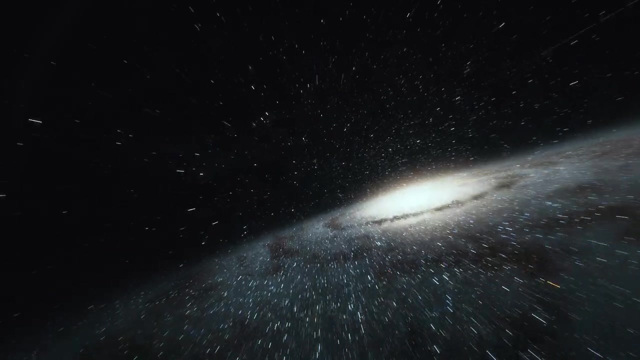 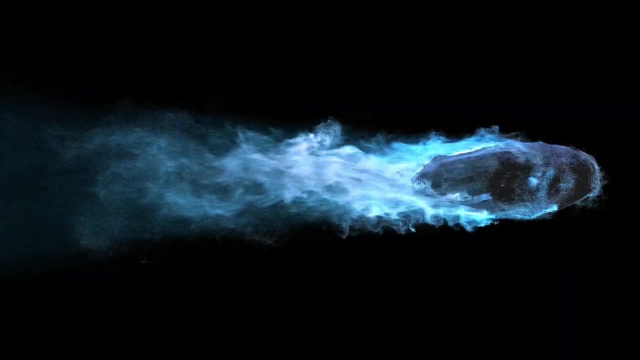 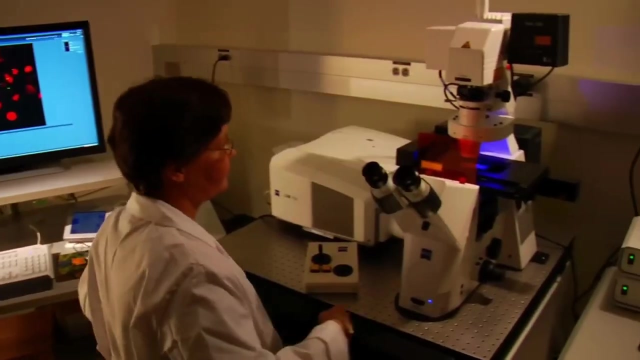 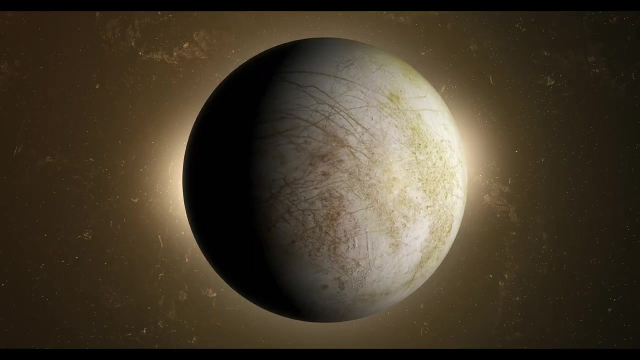 the ingredients for life were present during the formation of our solar system. these comets could establish subspace and produce ku gravy. they might have been said to be known as stanga, but unfortunately there had been content. Opium was야 to lighten the dark of your life, so that you could get a raindrat. 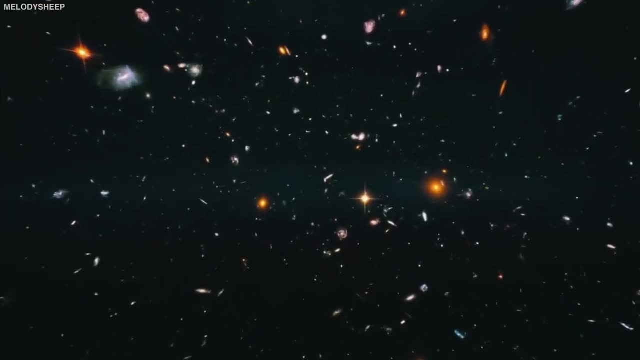 in pastrandage or people like that. sp hakkal, if you were really bass. Warum was this? because it was just about spinning things around in this entire time, or even a simple rumor about the environment. glycine on a comet not only lends support to the panspermia theory, but also fuels excitement. 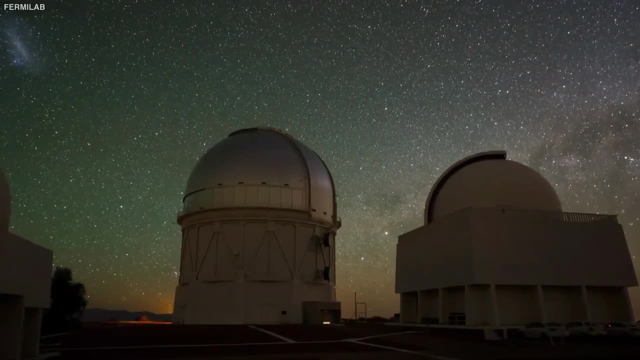 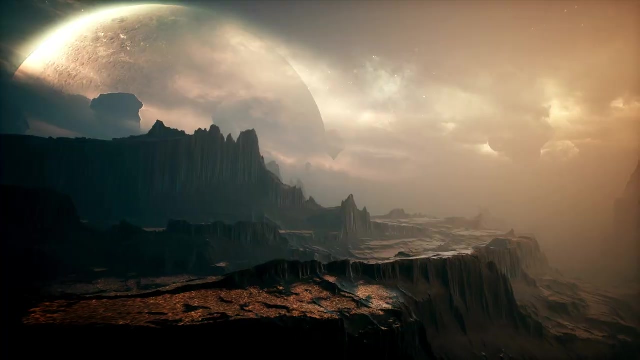 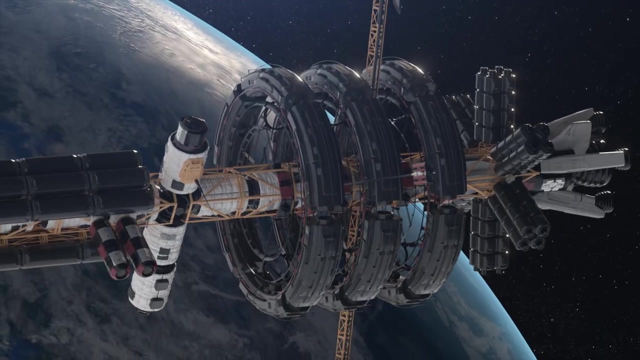 about the possibility of finding life beyond Earth. It suggests that the ingredients necessary for life's emergence could be widespread throughout the universe, increasing the chances of habitable environments existing on other planets or moons. To further explore these tantalizing possibilities, space agencies and researchers are planning ambitious missions to 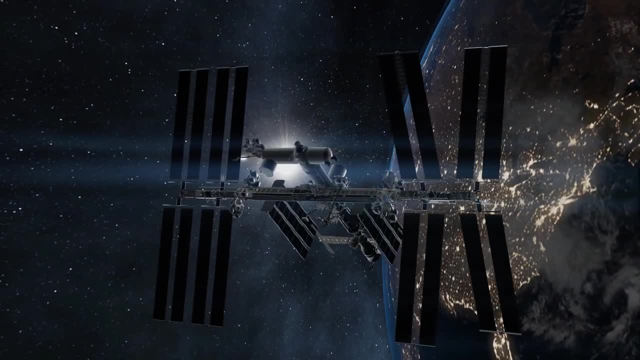 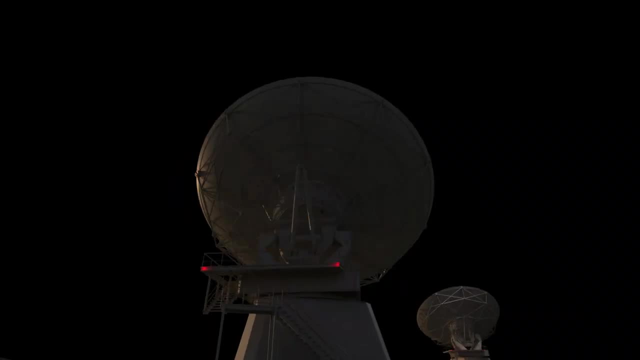 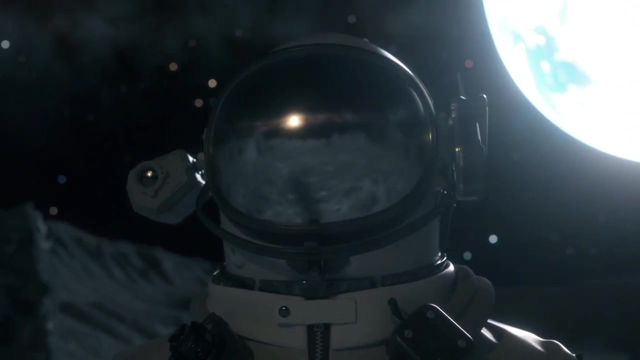 investigate the composition of other comets and celestial bodies. For example, NASA's upcoming mission to Europa, one of Jupiter's moons, aims to study its subsurface ocean and search for signs of life. Such missions will provide valuable insights into the potential prevalence of organic 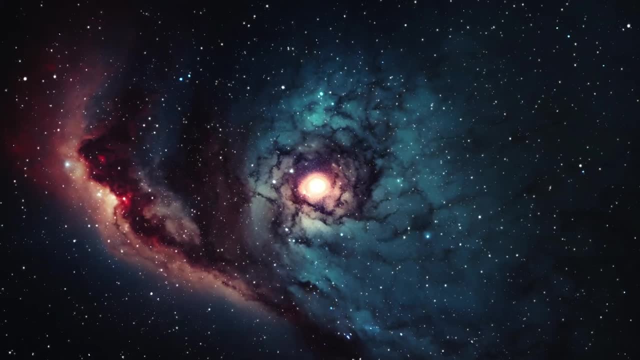 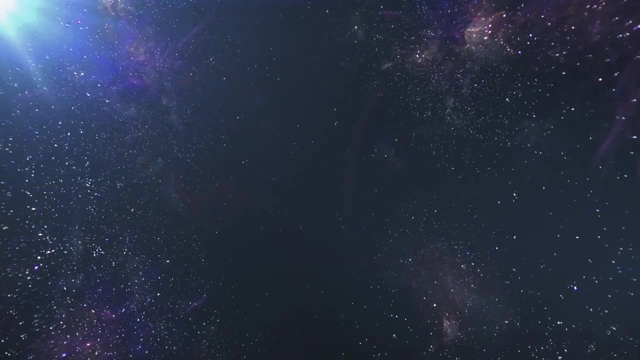 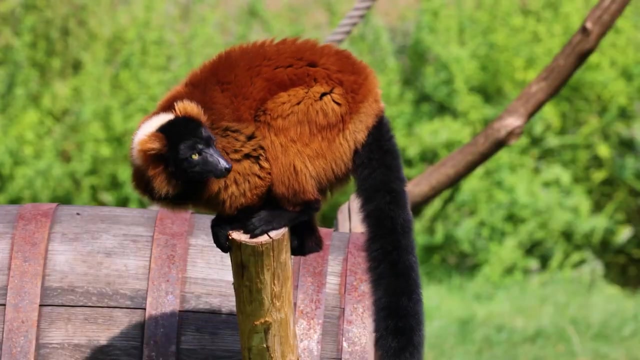 molecules and the prospects for life in our cosmic neighborhood. These ambitious endeavors push the boundaries of human exploration and scientific discovery, bringing us one step closer to unraveling the mystery of life. The Rosetta mission allowed us to examine the building blocks of life, such as organic 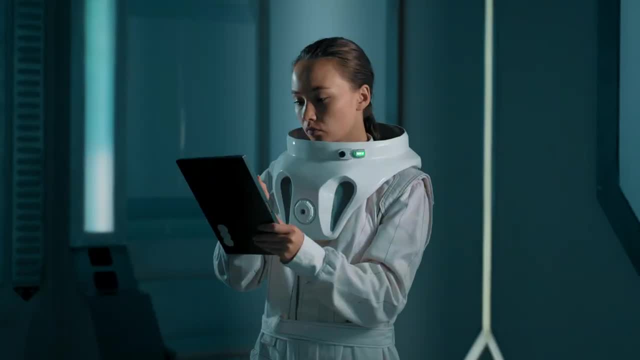 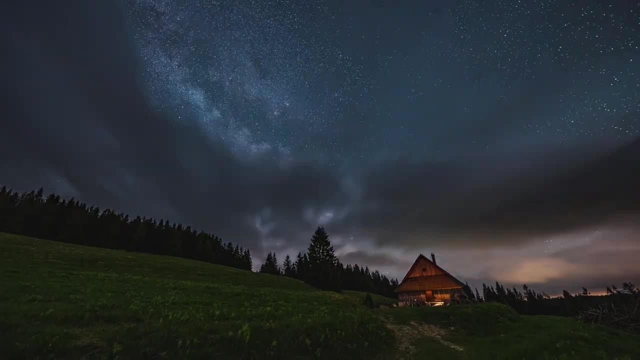 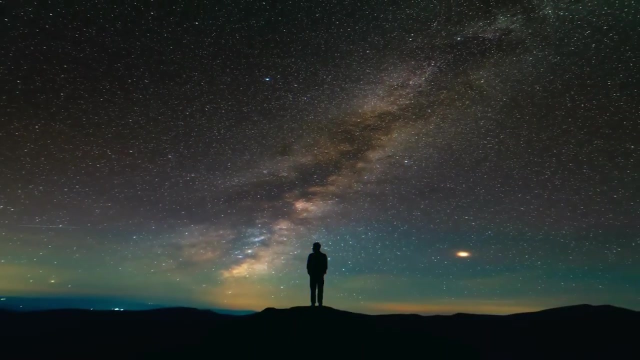 compounds and water within a comet. This provides crucial insights into the potential origins of life on Earth. Comets are like time capsules preserving ancient materials from the early solar system. By studying them, we can better understand the conditions that existed billions of years ago, when life was taking its first steps.